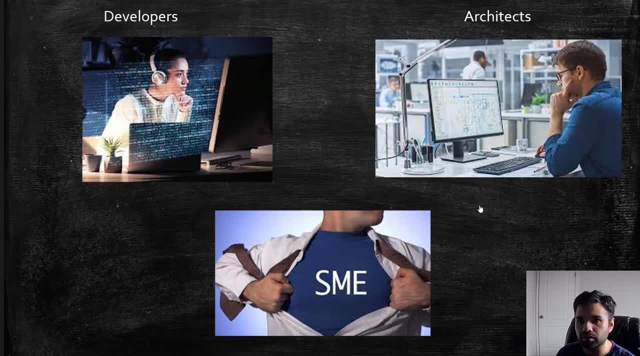 architects, because they know the architecture of the like. you know the application or product, whatever you're looking at, better than anyone else. and then you need subject matter experts, and when I say subject matter expert is there are in many organizations, especially large one, the authentication is very centralized. and there are organizations especially large one, the authentication is very centralized. 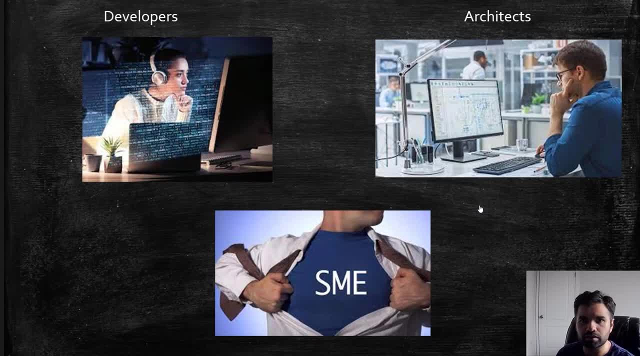 authorization is central module across many applications and they take care of that authentication authorization. so that's where you need to get in touch with this SMEs and understand this. like you know, critical components of the application, because you are not going to review everything manually. we discussed 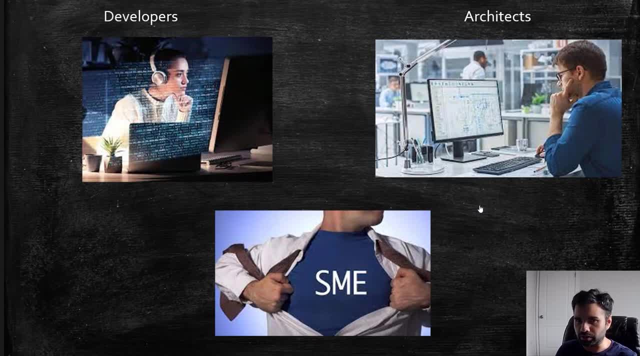 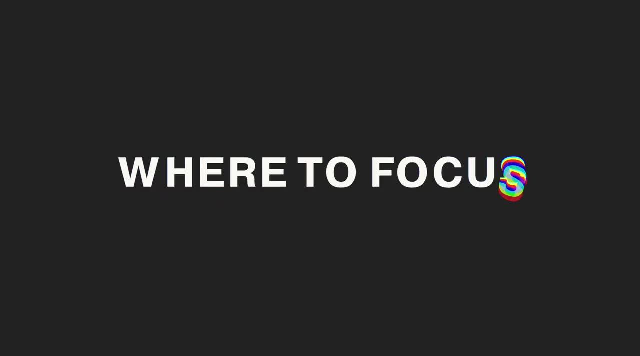 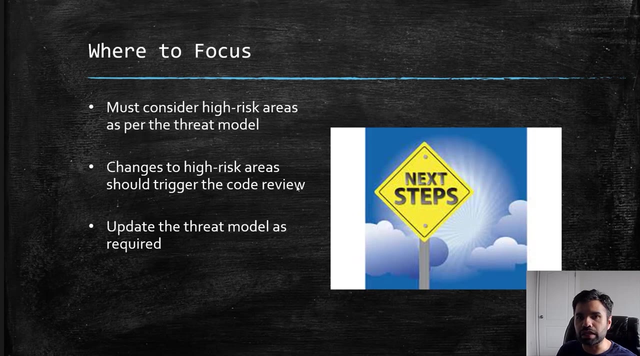 that right. so there are only a few components which you want to discuss or review manually. so that's where this SME is going to help you out. so that's that's one. now, where do you focus? like you know, where do you start, so you obviously want to start when you discuss with this SMEs architecture and 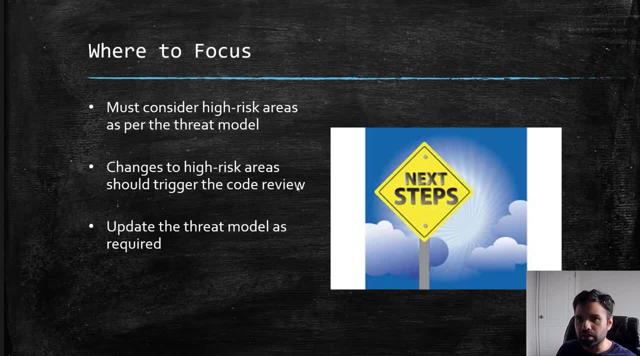 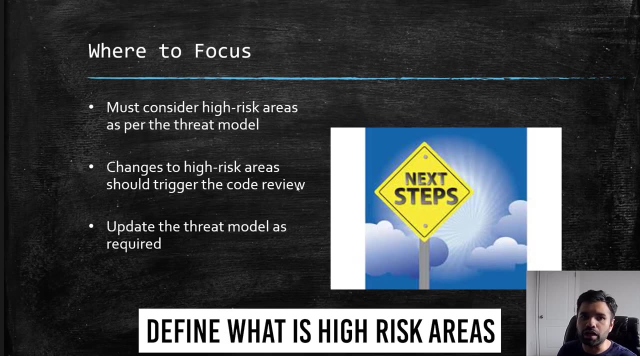 developers. they all have their own perspective. one person will say X is more important from their perspective. architect would say something else, SME would say something else. you need to collect all of this and then create like you know from your experience, from your expertise, define what the high risk area. 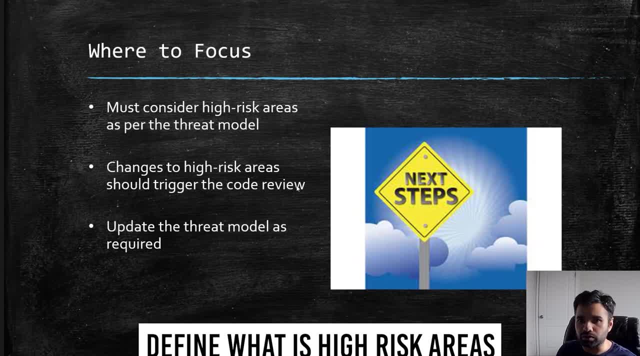 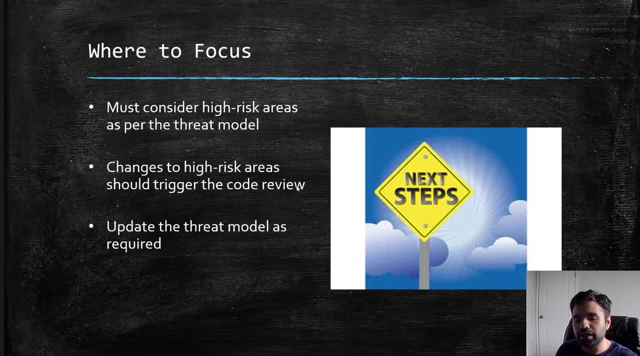 is, and then you might all of these and then create, like you know from your experience, from your also get a chance to look at the threat model for that. so once you have that, then also make sure when you're, when you are chatting with the developers, tell: 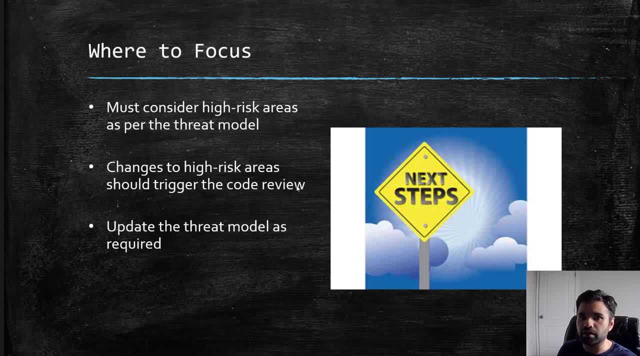 them like if you are making changes to any of this area. like you know, let us know, as a security reviewer, you should be reviewing the code, because let's authentication is working fine today, but after, in the next release, someone made changes to the authentication and now it is broken. so you want to make sure this. 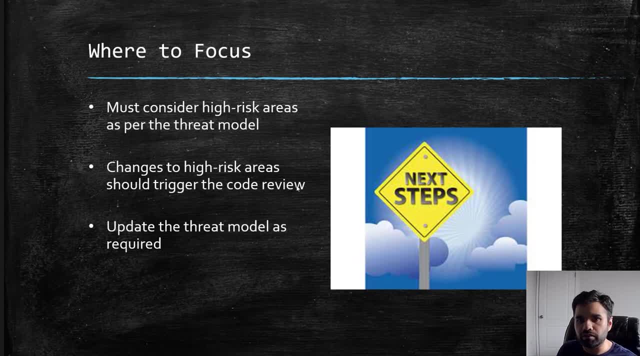 high-risk areas are definitely reviewed. and then when, whenever you are reviewing the code, whenever you find something interesting, make sure you you also update the threat model so it's easier when you do the next time or someone else is doing the code review instead of you. so let's take the risk based. 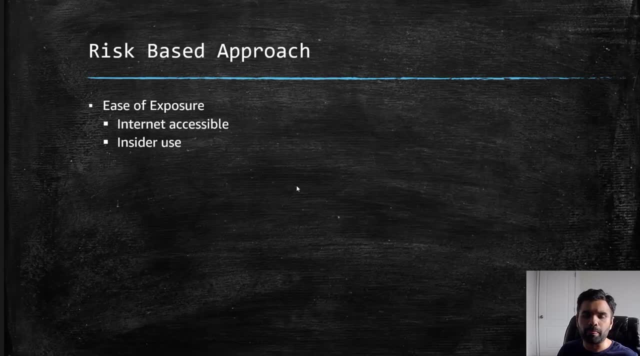 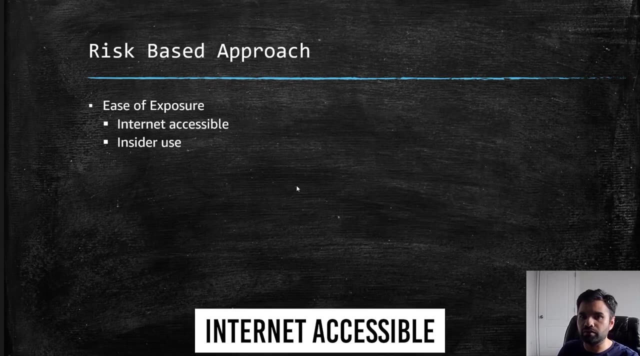 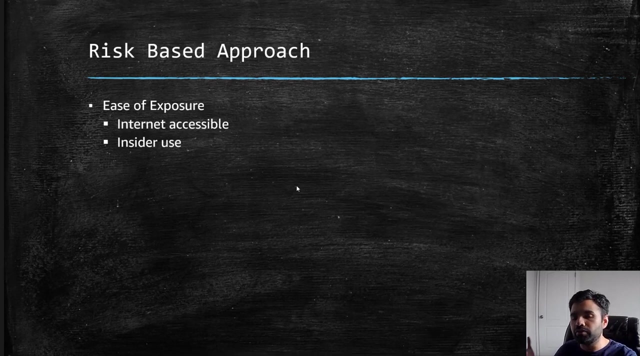 approach when I say risk based. first you want to find out, okay, which of these features or components are going to be internet. internet accessible, like you know, maybe login screen is something which everyone in the world will be able to see if your application is on the internet. but other features? 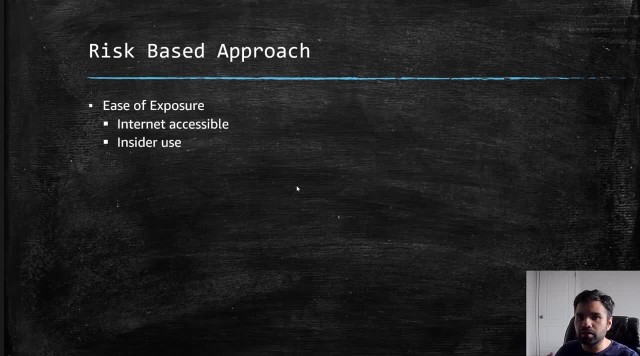 which is behind the internet, behind the login screen, will not be accessible. so it has, like you know, limited exposure. it still has high exposure if the authentication is broken, of course, but otherwise it has limited exposure. so you want to focus on the first. like you know, what are the internet accessible pages? 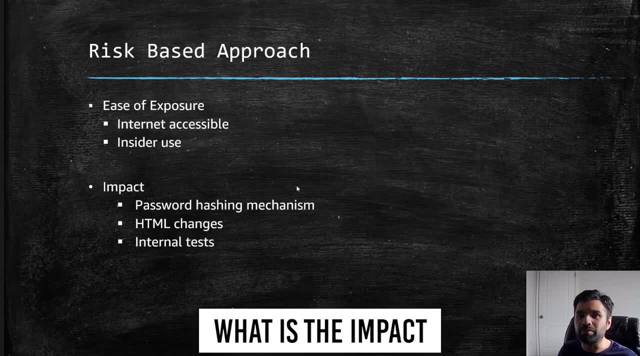 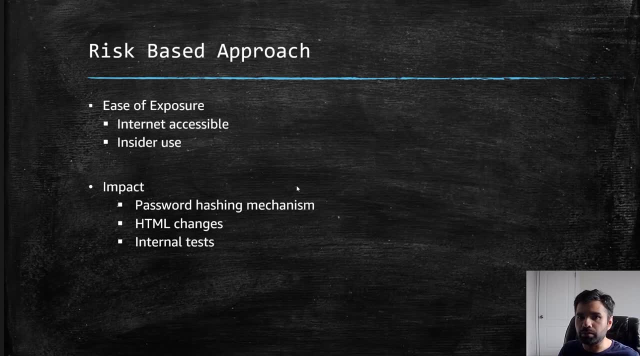 or features. next, you want to see what is the impact. the impact differs from like computer application or a computer application, but it is very important to compare and I hate to go back to the same example. but suppose, like you know, your, your password is compromised and that has a huge impact on your customer. 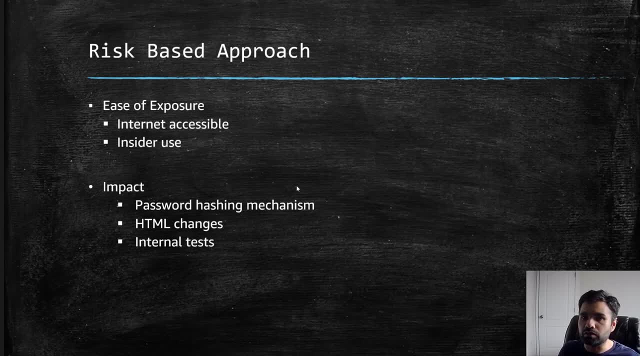 let's say you are not using the proper hashing or whatever. the scenario is, salt-and-paper technique is not working as expected. so then your that impact will have, like you know, a very, very huge on the customers, versus if they're, like you know, somebody is able to do the HTML injection or some. 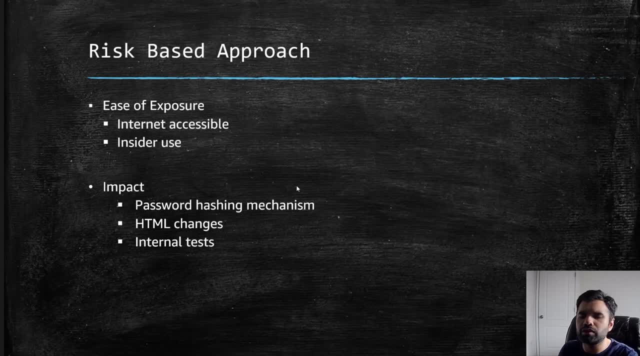 and it's not. it is wonderful, that's fine. it only has access to the test data, so we don't, we don't anticipate, like you know, much impact. so so see which one is the high-risk area from this, this methods, and sometimes you also have like. 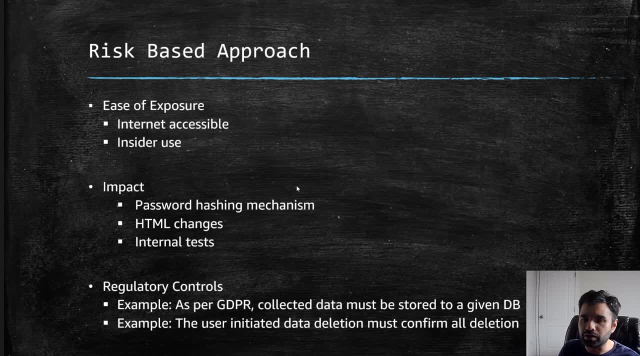 you know, compliance requirement, depending on which country and where this product is going to be hosted and used. but as for the GDPR, for example, collected data must be stored to a given database in a certain location. now, when you're doing the code review, you want to make sure, like this code, this data. 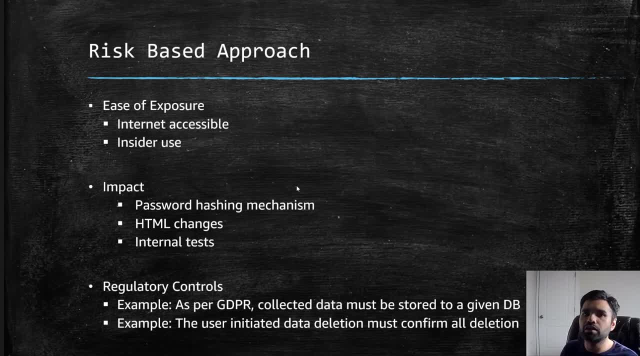 cannot go beyond, like you know, Europe region, for instance, or sometimes there is a requirement that it must. like you know when, when customer says I want to delete my data out, I do, I want to delete my account, then that deletion should go through and delete every customer data from all the database. so these are some. 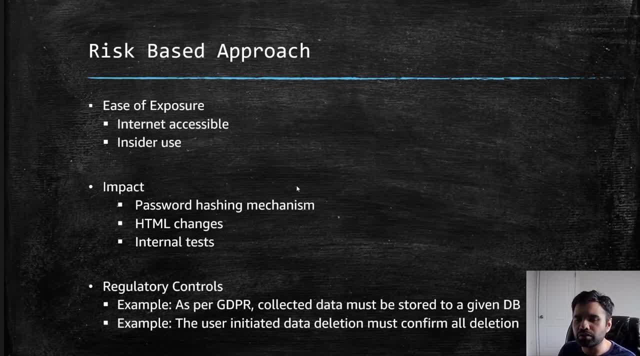 of the compliance checks that you also want to review manually? I don't think so. any tool, SAS tool, would cover all of this. they don't even have knowledge on like in all this requirement. so there, they cover like 70, 80 percent of the task, but 20 percent we. 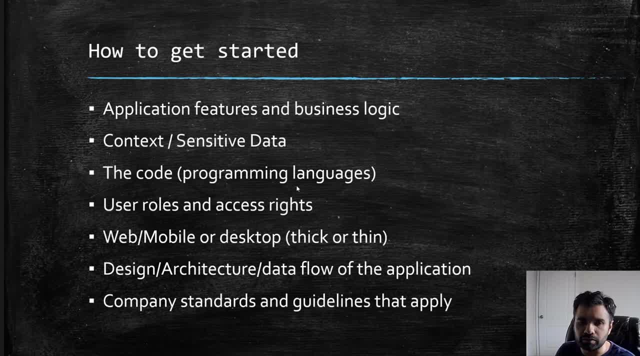 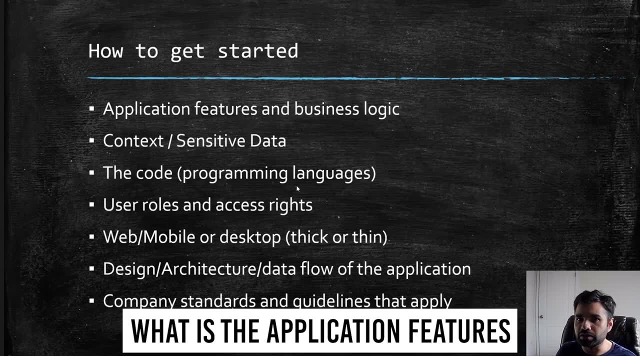 have to do it manually and that is where, like you know this, this guide will be helpful. so how do you get started? first of all, you want to understand what the application features are. business logic. this is similar, I think, what I said in the threat model as well. so when you do threat model, you want to 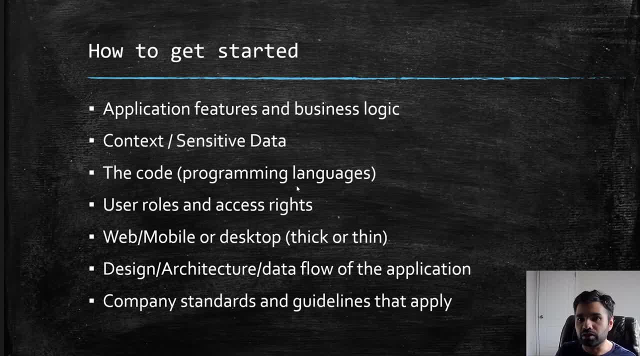 understand the same thing. then you want to understand the context or the sensitivity of the data, like maybe some data is sensitive, some data is not, some data is classified, some or not. so you want to understand like which components handling the data and everything. then you want to understand: 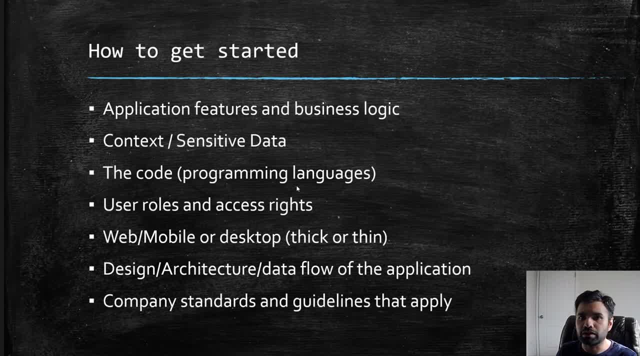 programming language, because you might not be aware or mastering all the programming languages that the core has written. there will be, like, a lot of, like you know, libraries. there will be a lot of front-end, back-end code, so maybe different framework, so you want to collect all the languages. This will also help you if you are running. 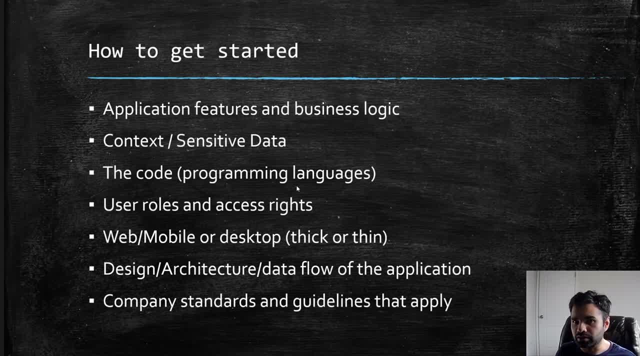 the SAS scanner, because not all the scanners are good at all the languages. User roles and access rights. this is also critical for access control authorization. You want to understand what are the user roles which are defined and, like you know, what permissions they get. So when you are reviewing, maybe you can review the, like you know, sample of. 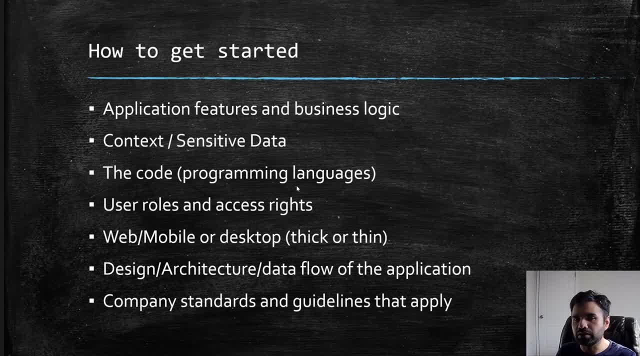 the code. You take one user, for example, like you know admin, and see: okay, is admin able to do XYZ activities as defined, or they can. there is also a way that they can do, like you know, some super admin kind of activities. Then you want to find out if it's a web mobile. 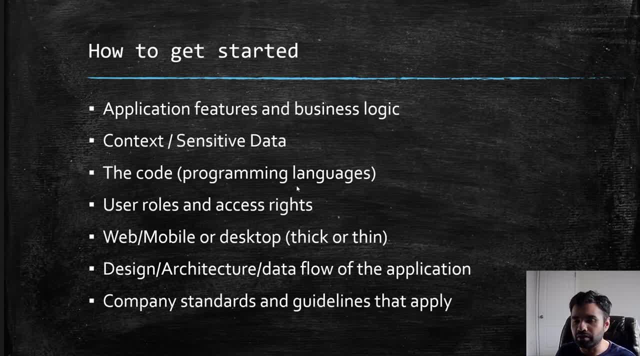 or desktop application- Thick client, thin client, right. that will differ a lot. If you are using the mobile applications, then you also want to talk about like: see how the code obfuscation is done, etc. Subtitles by the Amaraorg community. 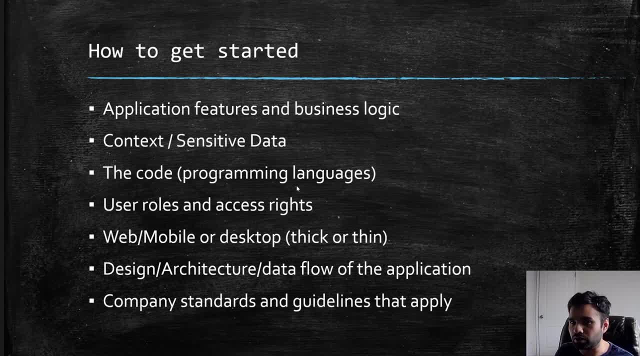 because that's very critical to the mobile applications, while web is not so much. So you want to, like you know, your test cases would differ from what kind of application that is. Then you also want to see the, like you know, design flow of application, because 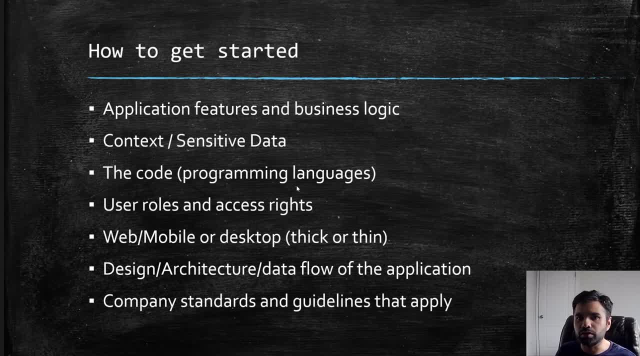 when you are reviewing the code. if you don't know the flow of the data, you will get lost in the code. And then, lastly, as we discussed, like you know, company standard and guidelines that apply. So if your company guidance, like the specific policy, that all the tools, all 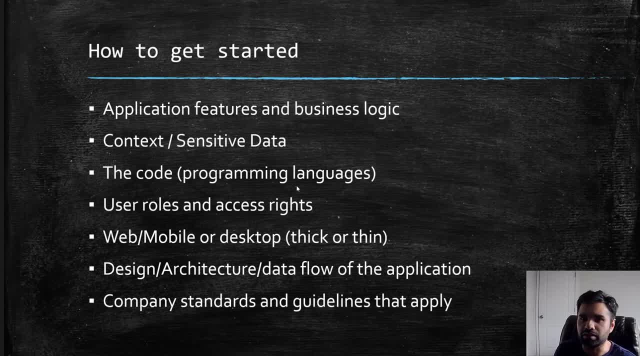 the applications must have 16 character of password right, Let's say that's a policy. So you want to ask the SMEs like: are there any such policy? and if so, you want to find evidence in the code if that policies are met or not. So this is another thing you want. 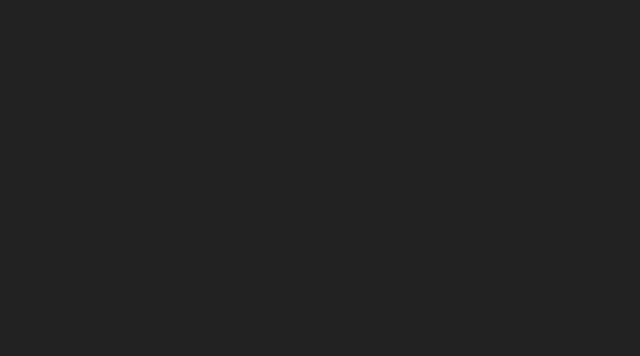 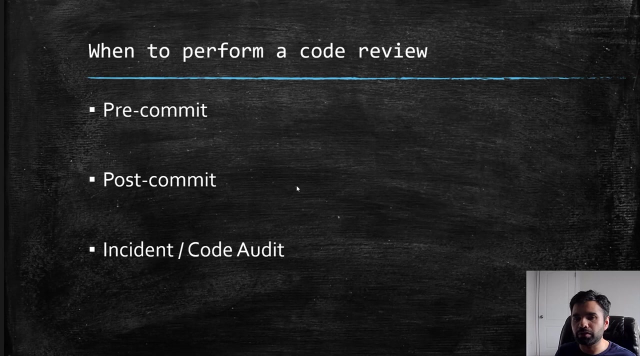 to. you want to check off, like when you want to get started with the code review. Now, when is the good time to perform the review? I think most likely. from my my perspective, it's always good to do it in the pre-commit, before it, like you know, goes to the market. 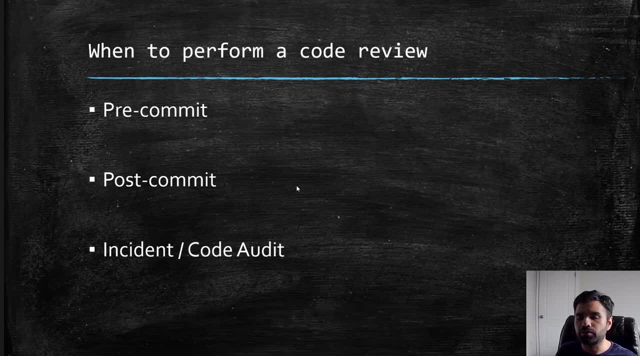 The master branch and, like you know, available to everyone. You want to find all the security vulnerabilities before you commit, So that's the best place. Sometimes it doesn't work that way, especially with the start-ups, like they don't have that much time to like you. 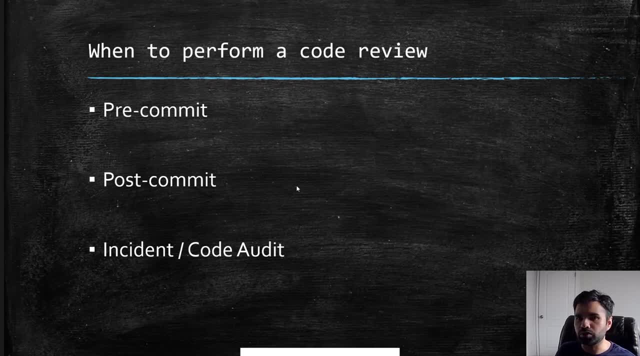 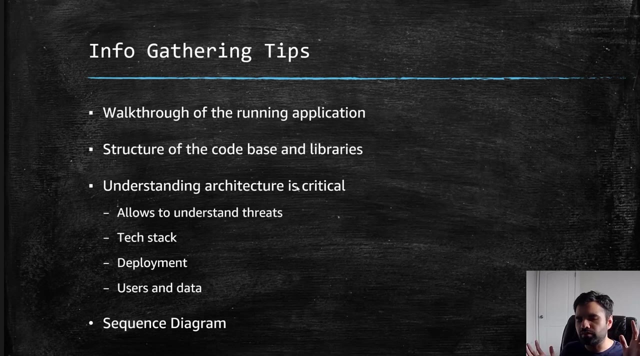 know, wait for the security approval. So then you do the like post-commit. But then there is also like an incident and you want to find out the root cause. then you definitely want to do the code audit. So then let's see, For the first step, like you know you want to, I told you like this is the information. 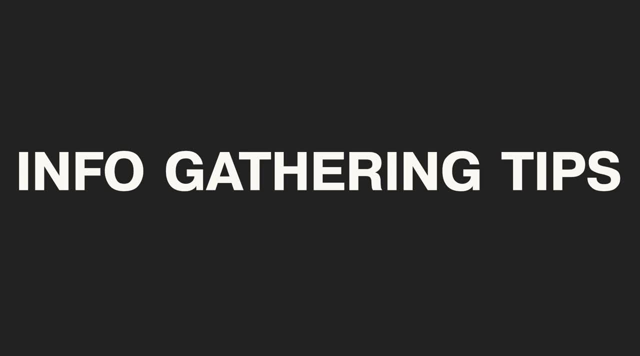 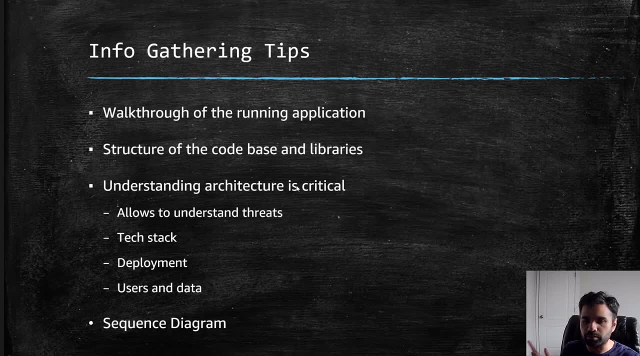 you need to gather. So how do you gather all this information? So first step you can do is: you can. you can just, like you know, sign up, ask someone to sign up for like a task credential, and you just walk through application yourself. This will give you a lot of information. 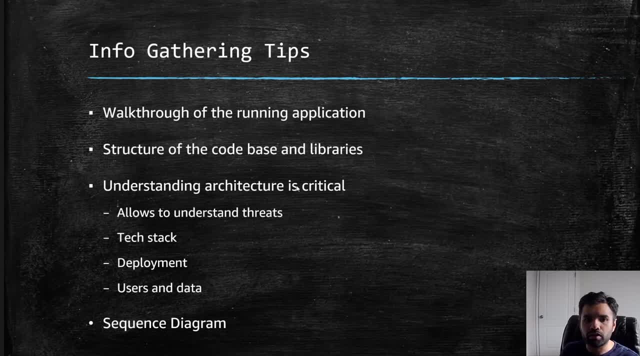 you can read through the documentation of the product. Then you can, like you know, you can download the source code and see how the structures and code base and libraries are structured. Then you want to sit with the architect, which we discussed in the first slide: You, because 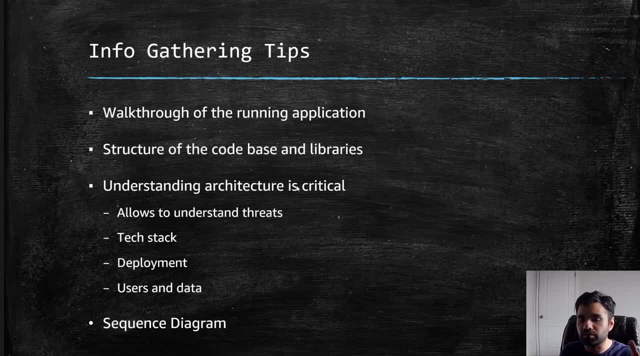 that will give you, like you know, understand the threat, like what's in the trust boundary, what's outside of trust boundary, which component is there, which component is coded in which library, etc. Then you will understand the tax tag, you will understand how the deployment 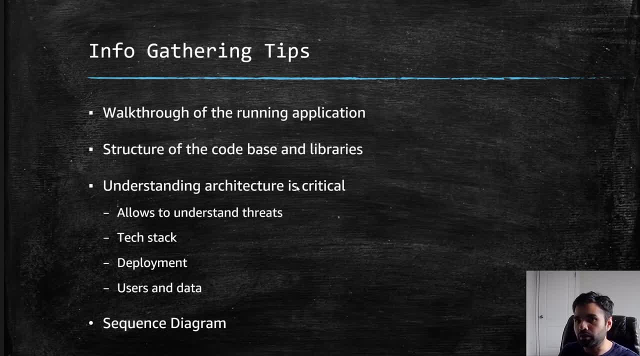 works, whether you should be able to do it in the pre-commit or post-commit, based on their sprint and agile methodology. you'll be able to figure that out And then you can see all the users and data. So that's the first step. Then you want to sit with the 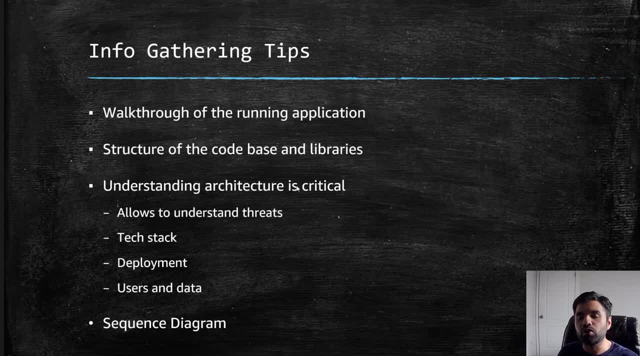 architect. so you have a list of all the users and then you have the equivalents and data that's stored in the different components And then, hopefully, if they have a sequence diagram for a critical use cases, make sure you ask them. that will help immensely to. 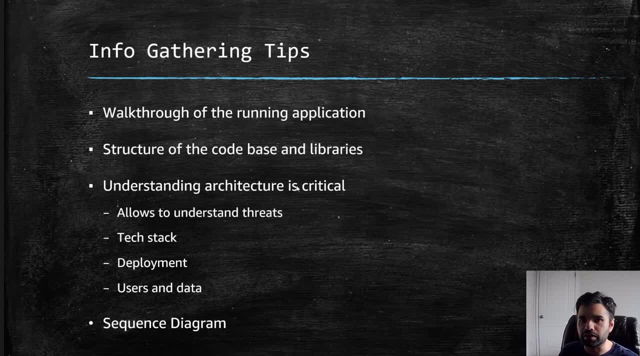 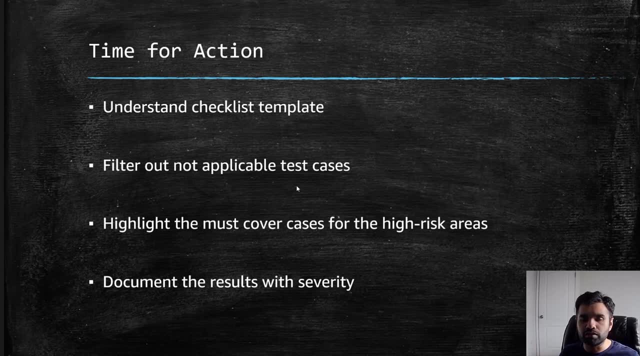 understand how each components are being used in the application. Now you gather all the information and now you are all ready to start. Of course, this steps. it sounds easy, but it's not. It's a lot of information you have to organize. 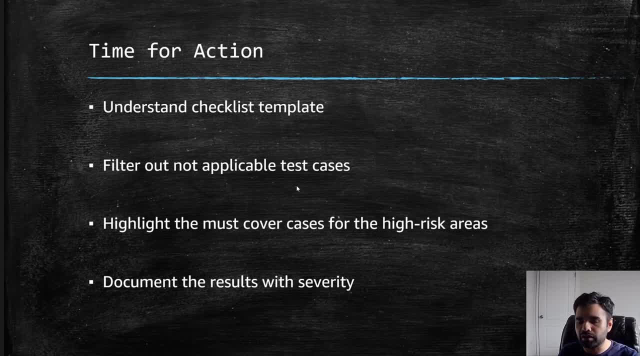 lot of things, So will get get through it. right, like as in when you do more code review, you will get to it. so then time for action. so what are the first of all? download and, like you know, create a checklist for what are the things that you're gonna do in the code review. you do not want to do 100. 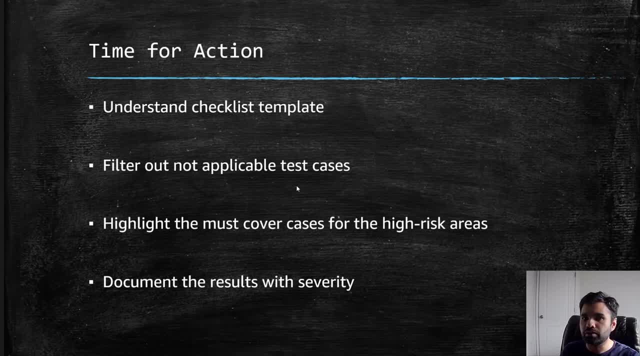 things. you do not want to check for 100 items, only the difference between what scanners are not not covered. or maybe the scanner you have does not support certain programming language, so you want to cover that. so make sure you you define that in the checklist you mark, like you know, which test. 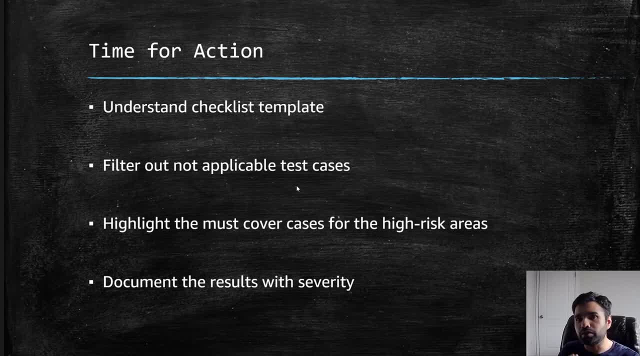 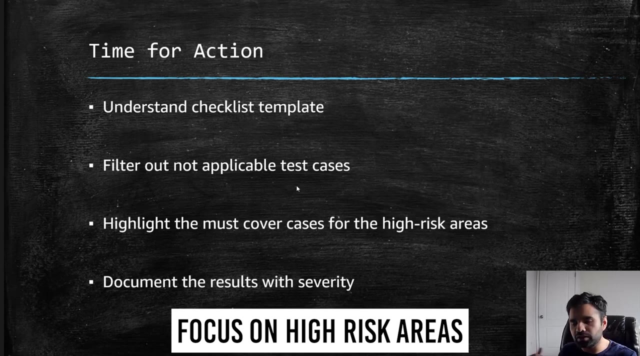 cases are required which are not. make sure you definitely take out those cases, like you know, which either uh is not applicable or probably is low in risk. you only want to focus on the which one is the high risk area and then finally, once you finish, go through all the checklists you want. 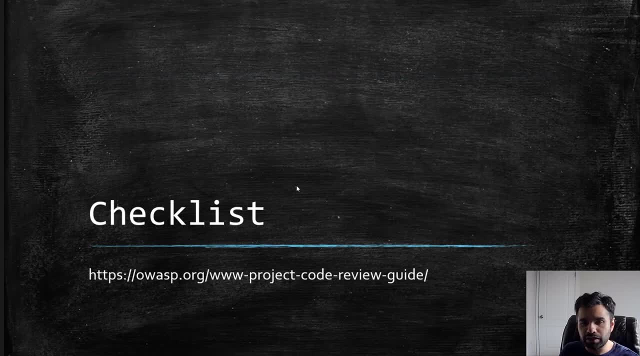 to document the result with the severity. now there is a really good checklist available. uh, also a guide. i would say uh. so this wasp guide is is very well in detail. it gives you the example on what the authentication i think, even if you are not looking to uh do like you know code. 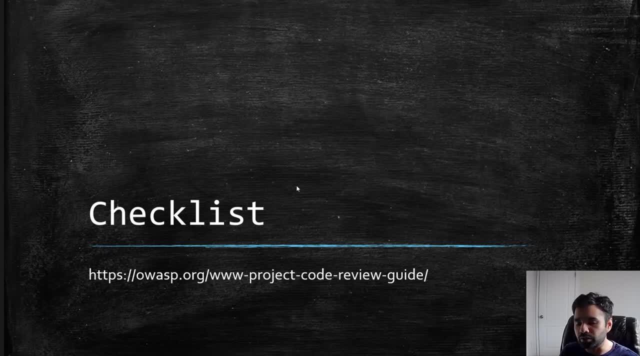 review or anything. just just read through the guide. i think it's huge. but even if you read like you know, uh, one section, like let's say you take one component, authentication, one area- and you just read through it, the example it's, it's going to immensely helpful, not just for the 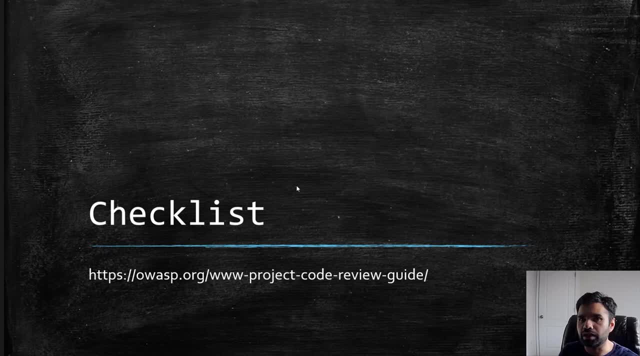 security, but also when you're, if you're a software developer and you're writing the code, uh, that's where also, it's going to be very useful. so i think, yeah, that's about it. i think i covered everything that i could think of. uh, what you need in order to get started for the code review guide. 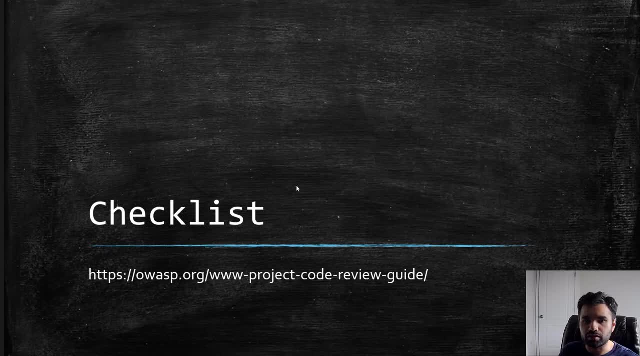 if you have any other uh suggestions or like you know, please drop it down in the comment. everyone would love to learn, even i. i would like to learn as well. if you haven't hit the like button yet, uh, please do it. this is, like you know, free content for you guys. um, also do let me know what other 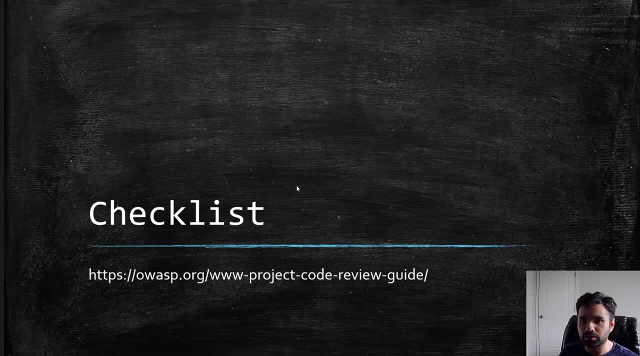 ideas, uh, that like topics you want to see in the future episodes, so i can, i can build my content accordingly. uh, and as well any other questions, feel free to drop it in the comment as well. uh. thank you all. i'll see you guys next week. bye.